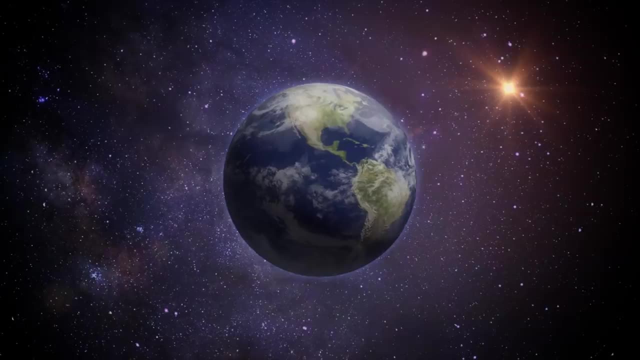 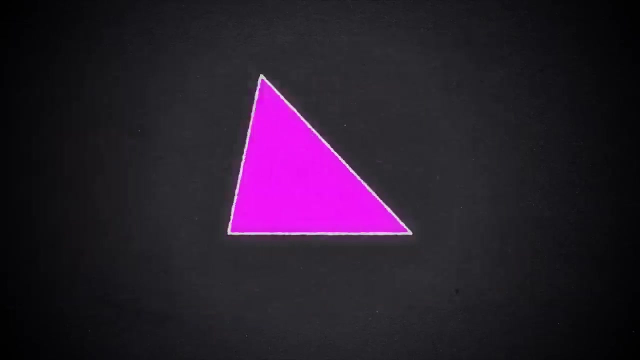 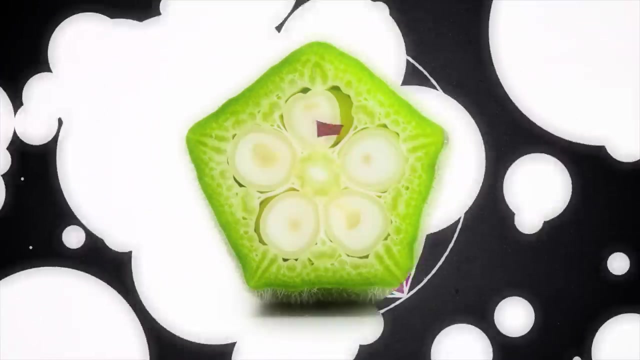 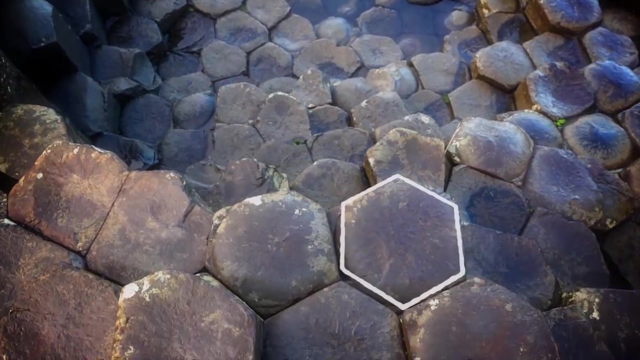 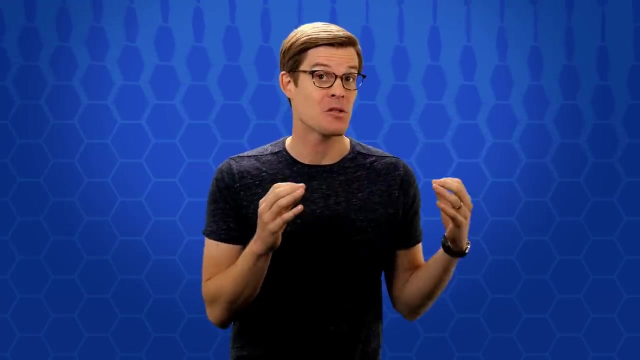 Is nature a mathematician? Patterns in geometry are everywhere, But nature seems to have a particular thing for the number six. Beehives, Rocks, Marine skeletons Insect eyes. It could just be a mathematical coincidence, Or could there be some pattern beneath the? 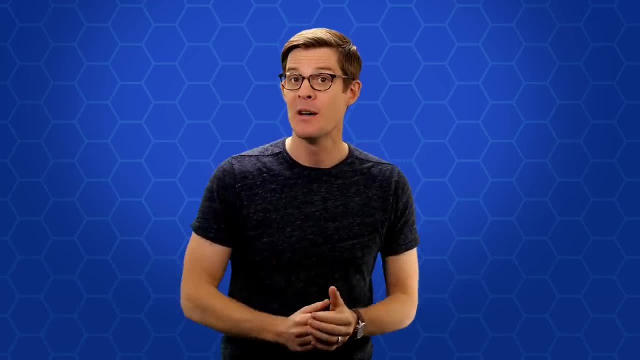 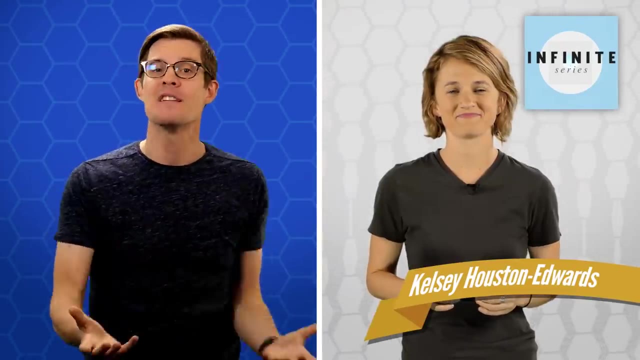 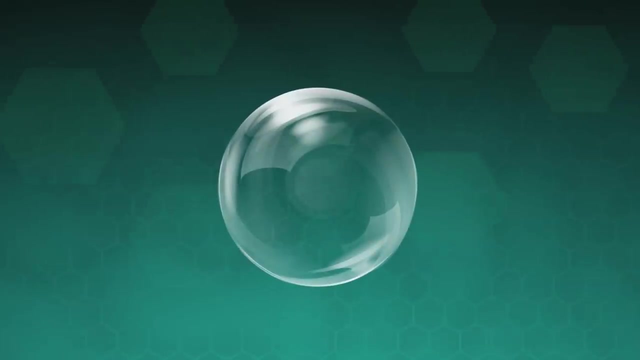 pattern Why nature arrives at this geometry. We're going to figure that out with some bubbles And some help from our favorite mathematician Kelsey from Infinite Series, Happy to help. A bubble is just some volume of gas surrounded by liquid. It can be surrounded by a lot of 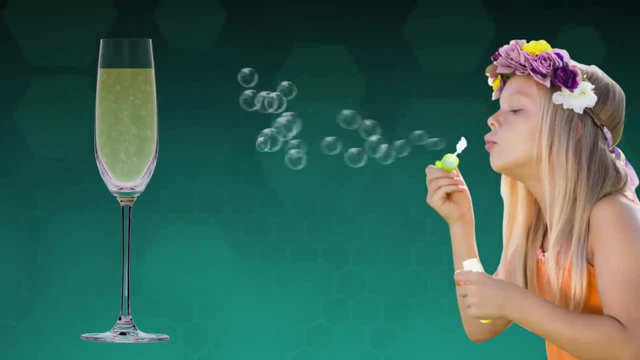 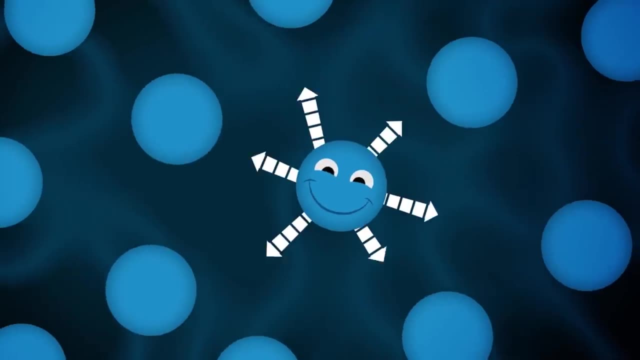 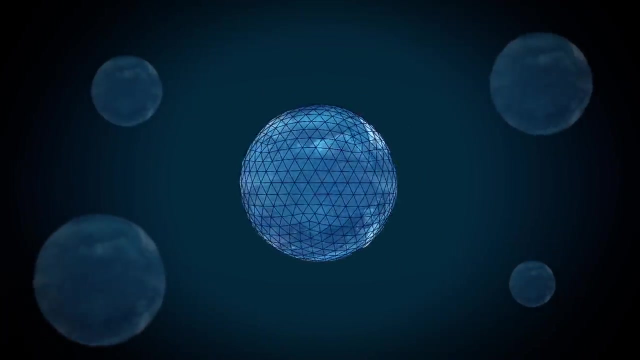 liquid, like in champagne, or just a thin layer, like in soap bubbles. So why do these bubbles have any shape at all? Liquid molecules are happier wrapped up on the inside, where attraction is balanced, than they are at the edge. This pushes liquids to adopt shapes with the least surface In. 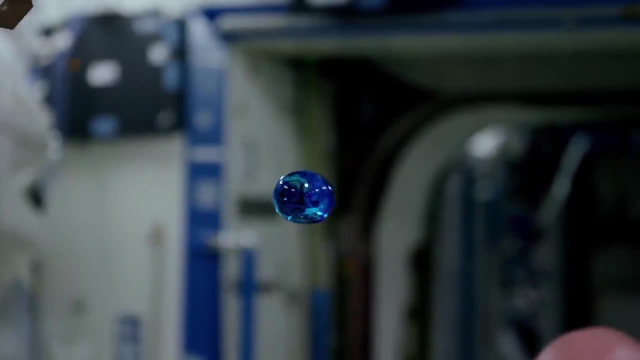 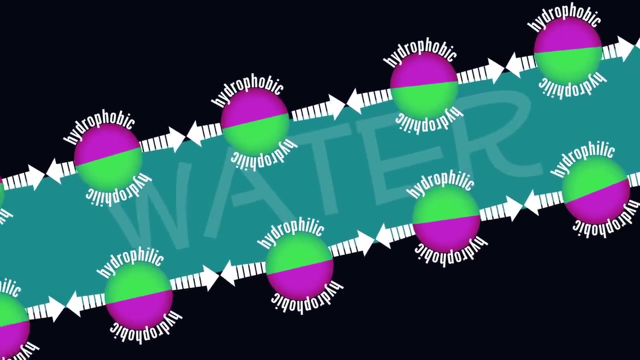 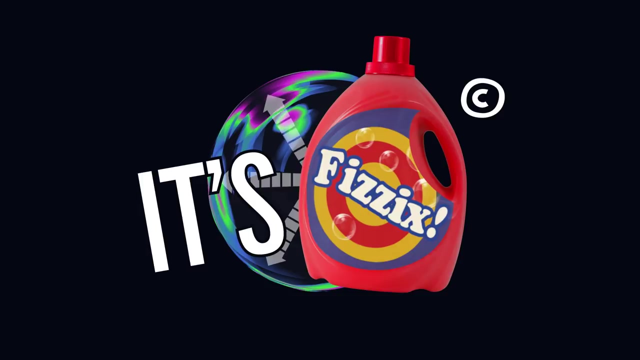 zero-g. this attraction pulls water into round blobs, Same with droplets on leaves or a spider's web Inside thin soap films. attraction between soap molecules shrinks the bubble until the pull of surface tension is balanced by the air pressure, pushing out. It's physics. 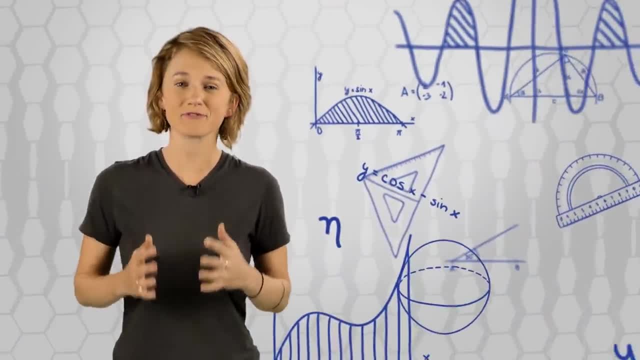 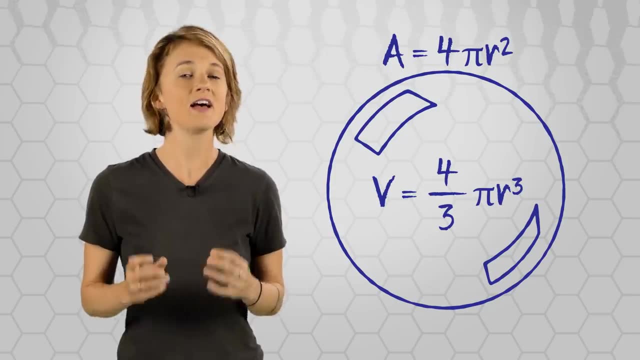 Physics is great, but mathematics is truly the universal language. Bubbles are round, because if you enclose the maximum volume with the least surface area, a sphere is the most efficient shape. Yeah, that's another way of putting it. What's cool is if we deform that bubble. 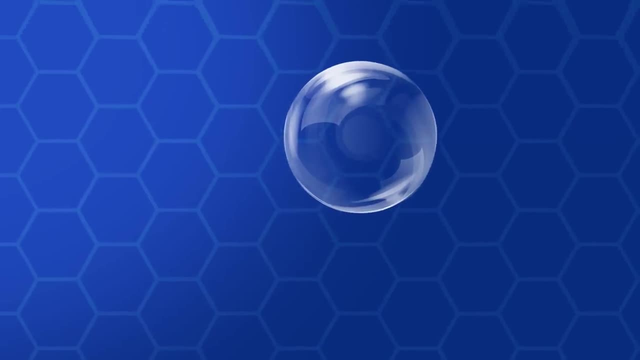 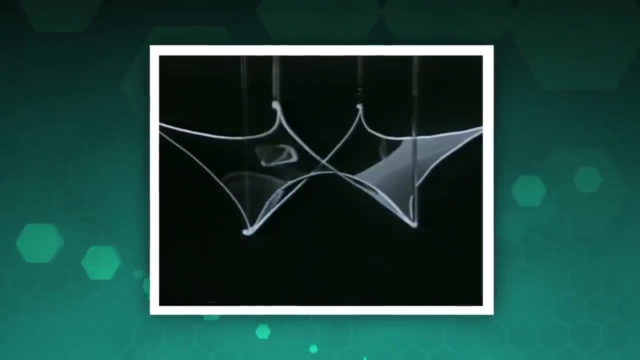 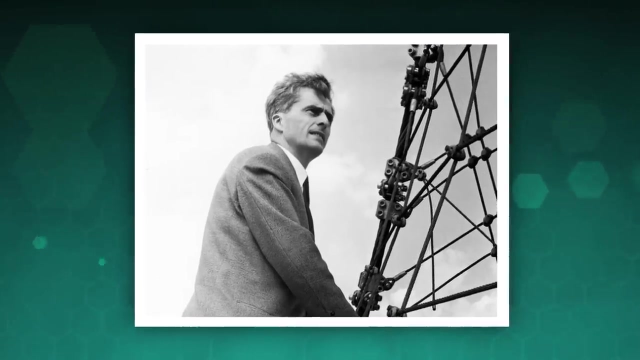 we get a sphere. The pull of surface tension always evens back out to the minimal surface shape. This even works when soap films are stretched between complex boundaries. They always cover an area using the least amount of material. That's why German architect Frei Otto used soap films. 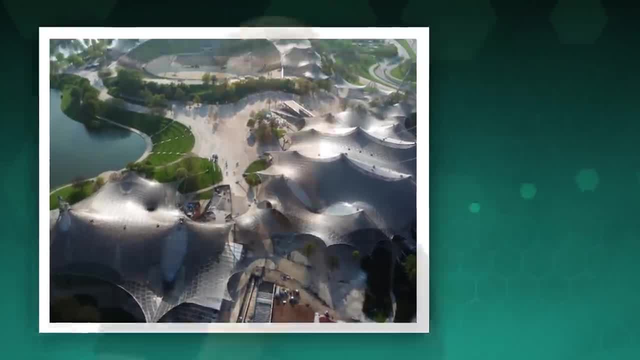 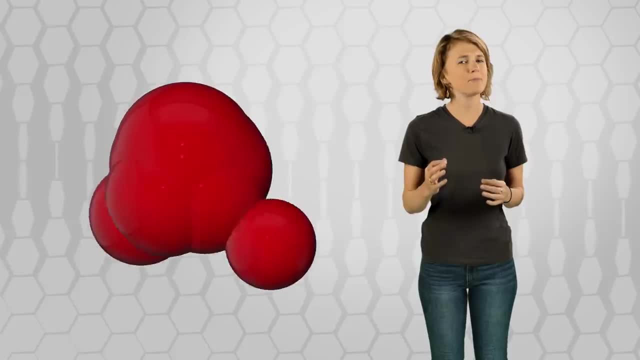 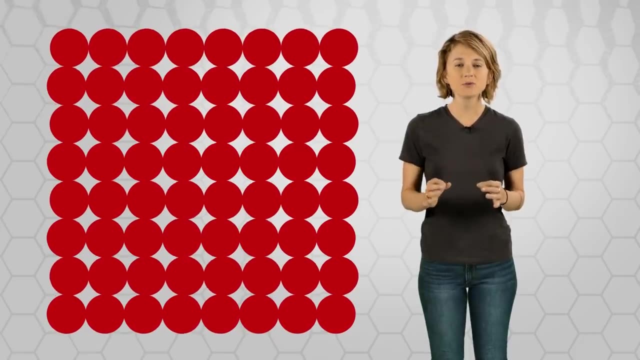 to model ideal roof shapes for his exotic constructions. Now let's see what happens when we start to pack bubbles together. A sphere is a three-dimensional shape, But when we pack bubbles in a single layer, we really only have to look at the cross section: a circle, Rigid circles of equal diameter. 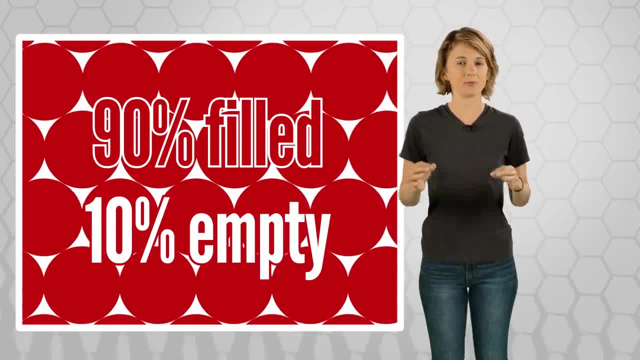 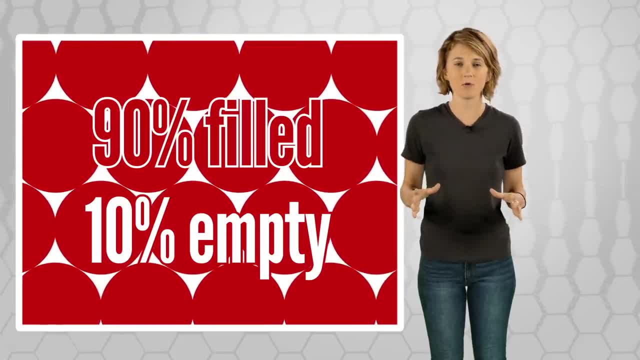 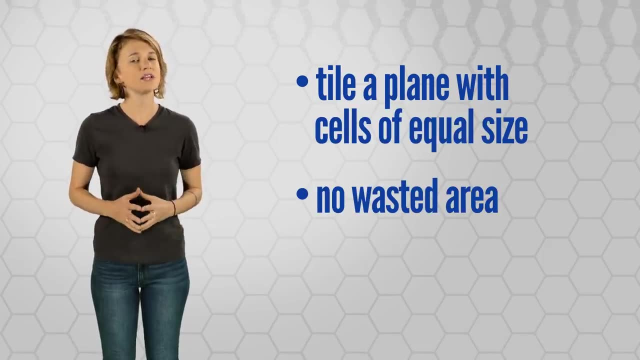 can cover at most 90% of the area on a plane, But luckily bubbles aren't rigid. Let's pretend for a moment these bubbles were free to choose any shape they wanted. If we want to tile a plane with cells of equal size and no wasted area, we only have three regular 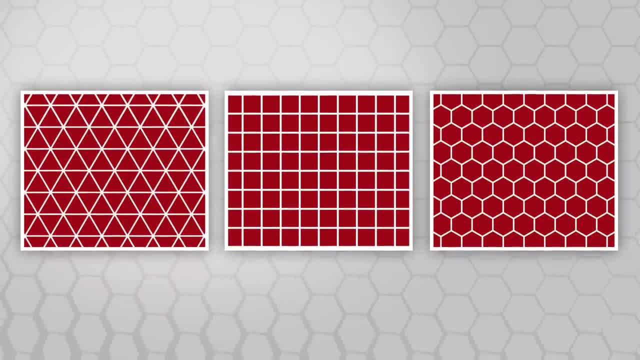 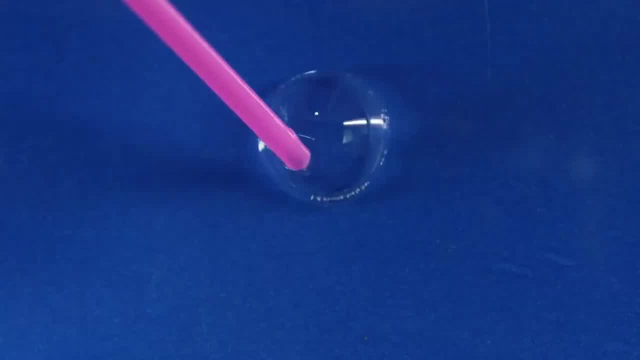 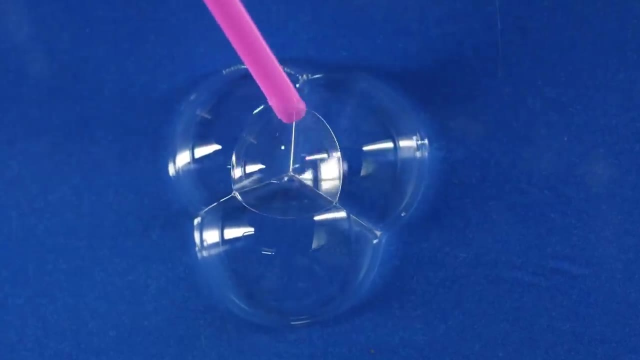 polygons, to choose from Triangles, squares or hexagons. So which is the best? We can test this with actual bubbles: Two equal sized bubbles, a flat intersection, Three, and we get walls meeting at 120 degrees. But when we add a fourth instead of a square intersection, the bubbles will always rearrange. 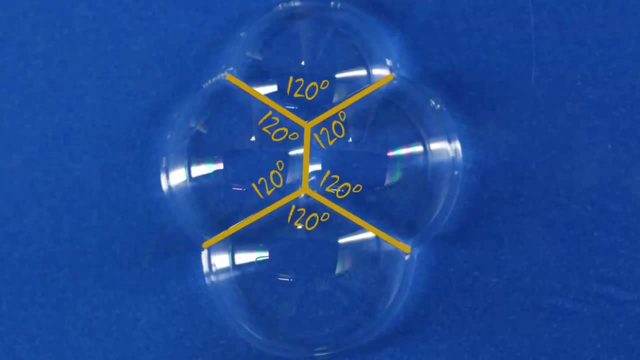 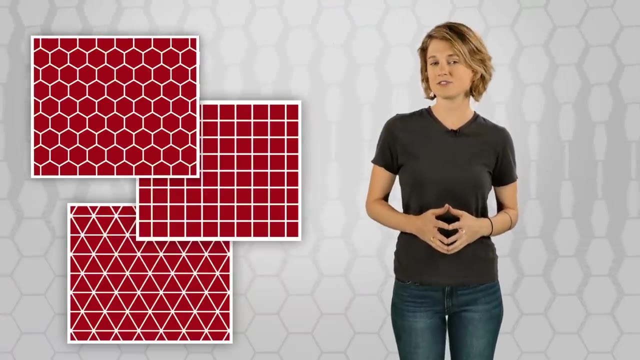 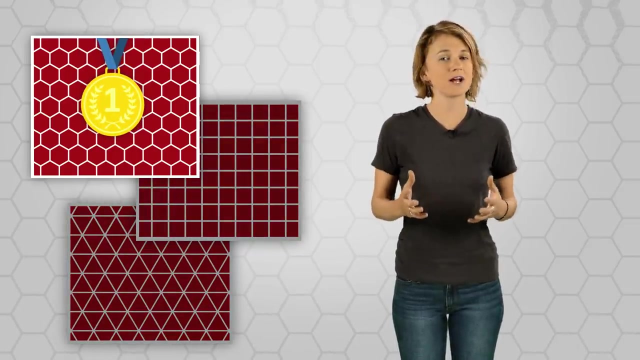 themselves. so their intersections are 120 degrees, the same angle that defines a hexagon. If the goal is to minimize the perimeter for a given area, it turns out that the hexagonal packing beats triangles and squares, In other words, more filling with fewer edges. 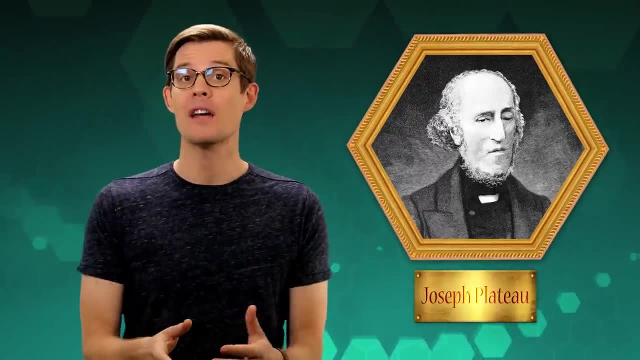 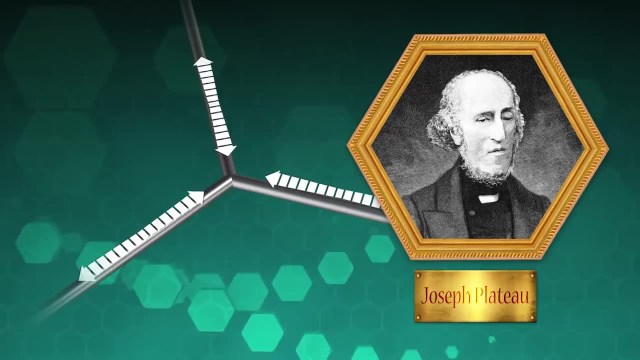 In the late 19th century Belgian physicist Joseph Plateau calculated that junctions of 120 degrees are also the most mechanically stable arrangement where the forces on the films are all in balance. That's why bubble rafts form hexagon patterns. Not only does 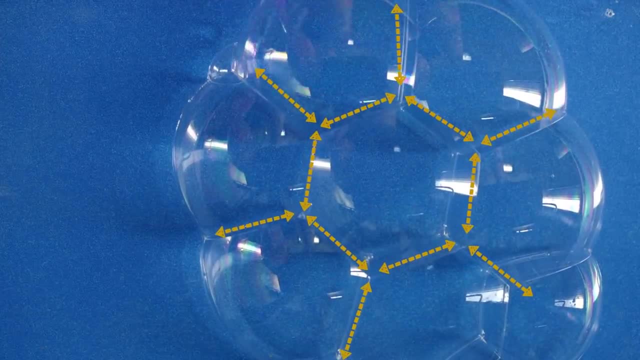 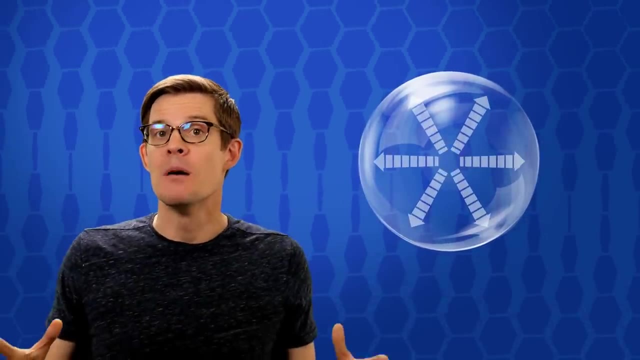 it minimize the perimeter. the pull of surface tension in each direction is most mechanically stable. So let's review. The air inside a bubble wants to fill the most area possible, but there's a force surface tension that wants to minimize the perimeter. And when bubbles 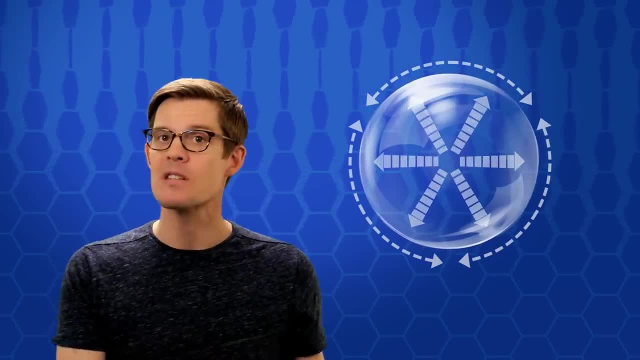 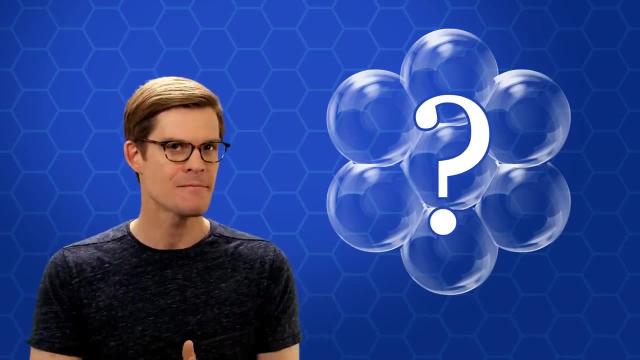 join up. the best balance of fewer edges and mechanical stability is hexagonal packing. Is this enough to explain some of those six-sided patterns we see in nature? Basalt columns like Giant's Causeway, Devil's Postpile and the Plains of Catan form from. 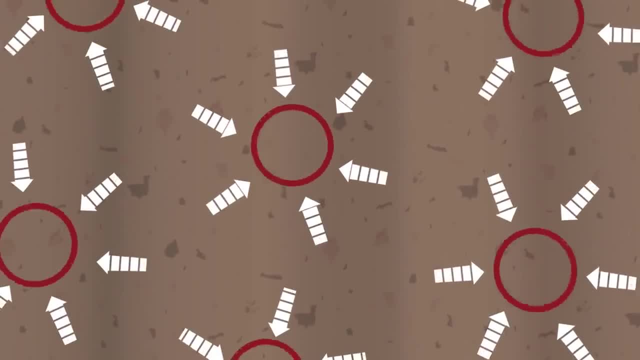 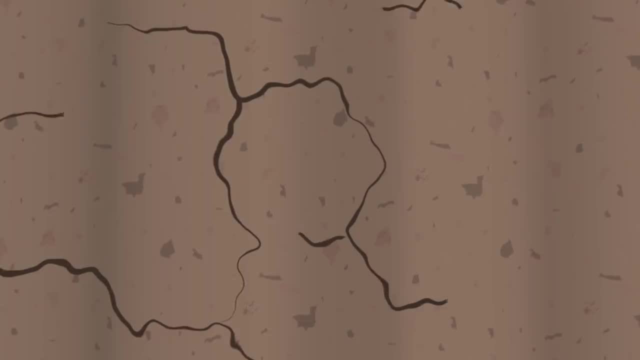 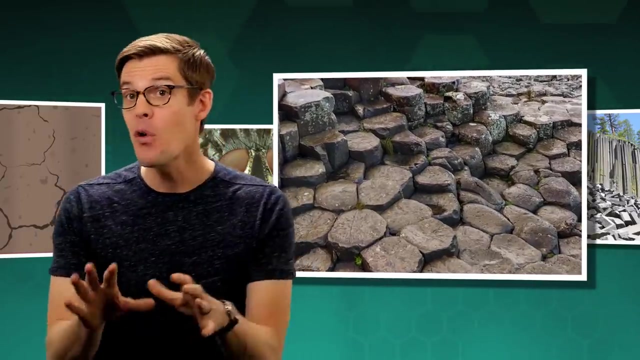 slowly cooling waves. Cooling pulls the rock to fill less space, just like surface tension pulls on a soap film. Cracks form to release tension, to reach mechanical stability, And more energy is released per crack if they meet at 120 degrees Sounds pretty close to the bubbles The forces are.